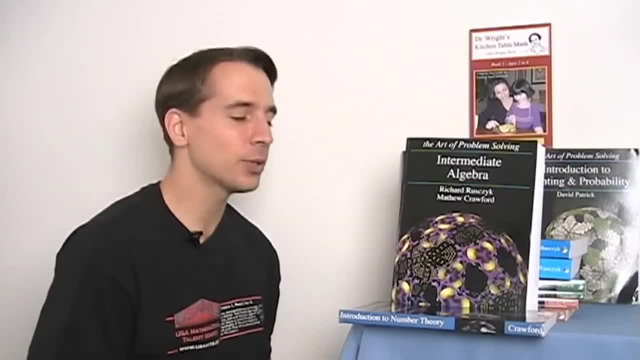 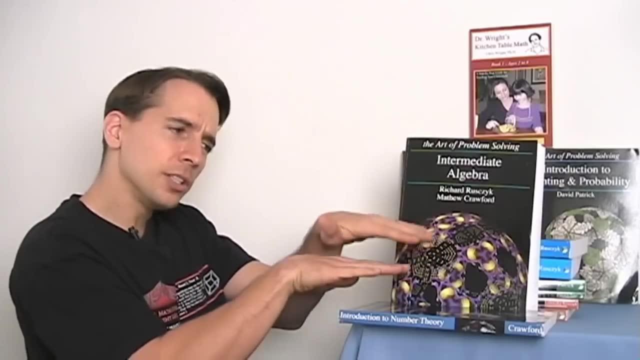 I shouldn't stack them up all like this and say, hey, look at these great books, look at these great books, They said. what I should do is I should just have three, just take three instead of all these and just, you know, subtly stack them up here in the front. 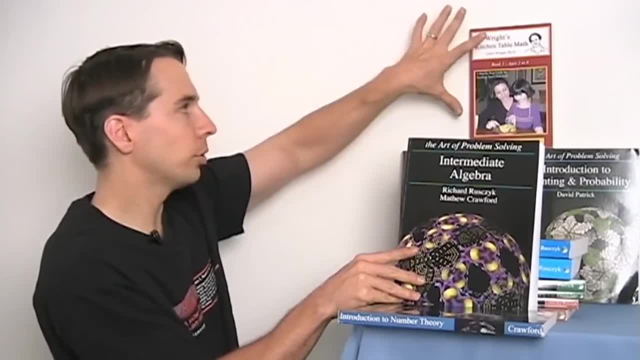 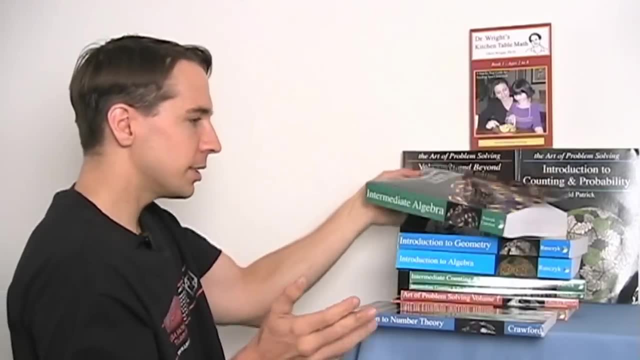 One, two, three. Not stand them up, like this great book here, or put them up on the board, like this one. So well, I don't know, it kind of pains me to do this, but I'm going to go ahead and take their advice. 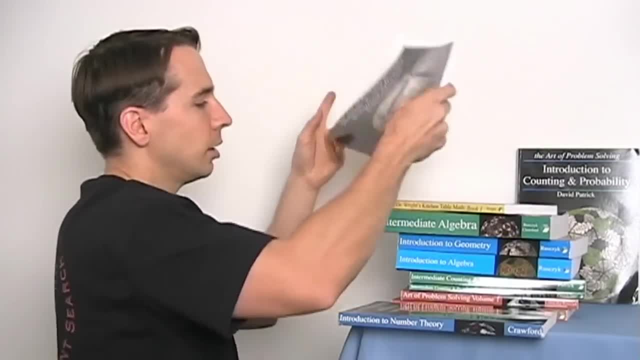 Besides, that will give me some more board space to work with. So I'm going to take these down and I'm going to pick three of these books and stack them up here And let's see how do I? oh wait. 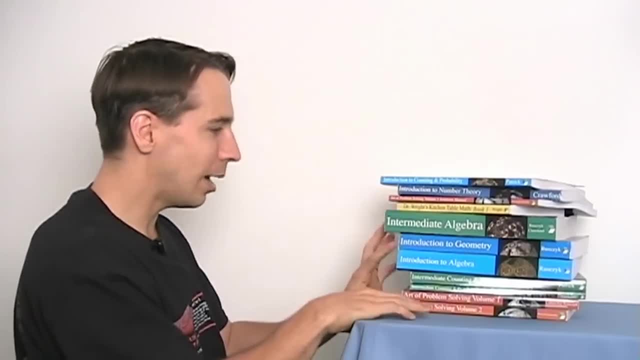 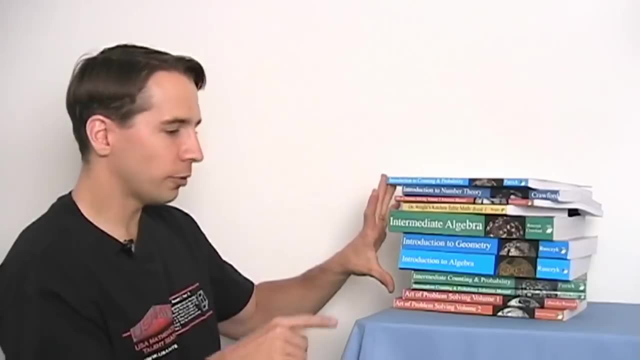 That's a math problem. The math problem is: how many ways can I take three of these books and stack them up here? That's a good problem. Well, we start well. first we have to pick the first book, the book that's going to be on the bottom. 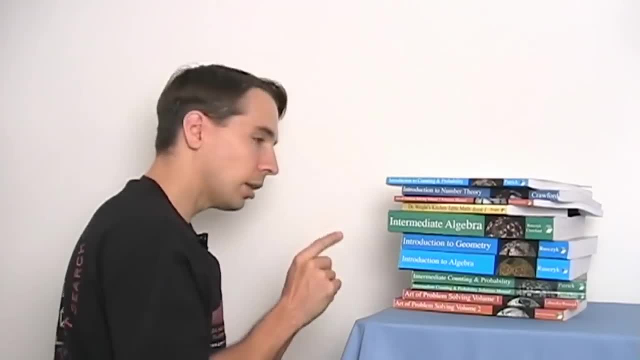 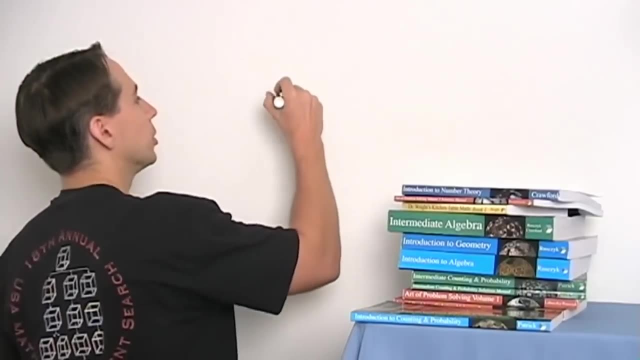 We'll count these. We've got four, five, six, seven, eight, nine, ten, eleven, Eleven books. So I have eleven different choices for the book that goes on the bottom. So I have eleven choices for the book on the bottom. 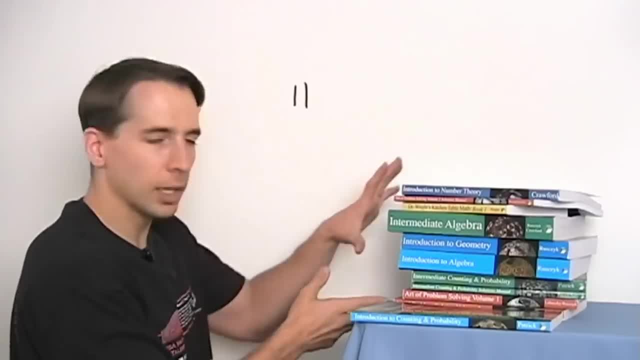 And then, no matter what book I choose to be on the bottom, well, there will be ten books left here, because I've taken one out of the stack already, And then I can just choose any one of them. There are ten ways to choose them. 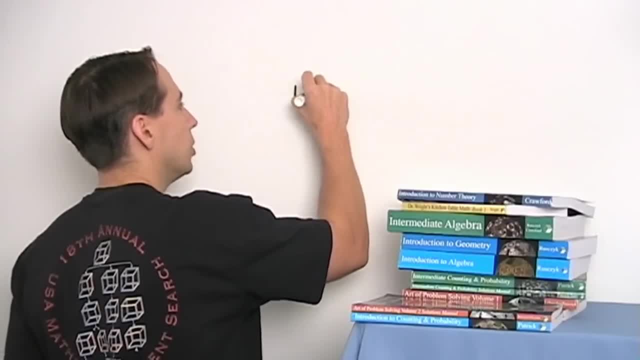 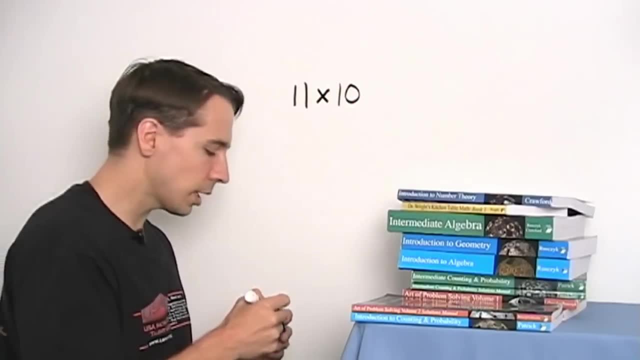 So there are eleven times ten ways to choose the first two books, Because no matter what book I choose first, for each of those eleven books there are going to be ten ways to choose the second book. That's going to give me different stacks. 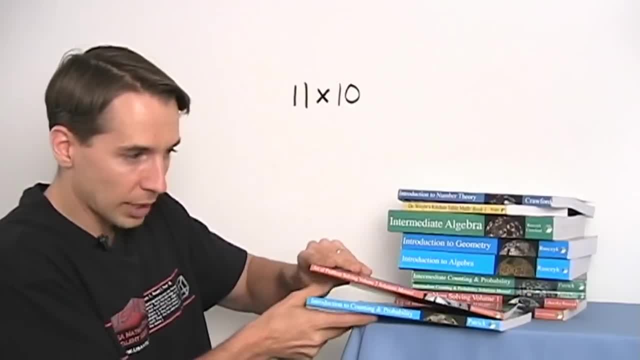 It's going to be a hundred and ten different stacks And again we care about the order here. You know, the stack that we have right here is different than this stack. It's the same two books. It's the same two books, but it's a different order. 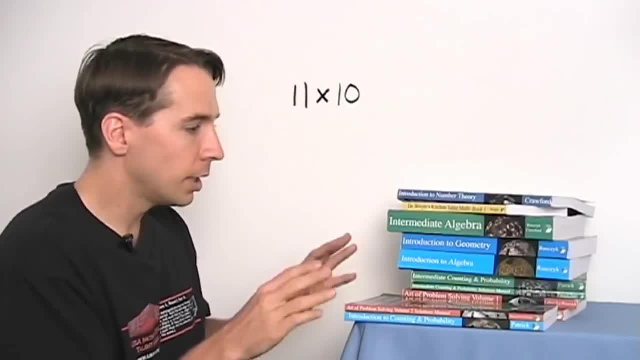 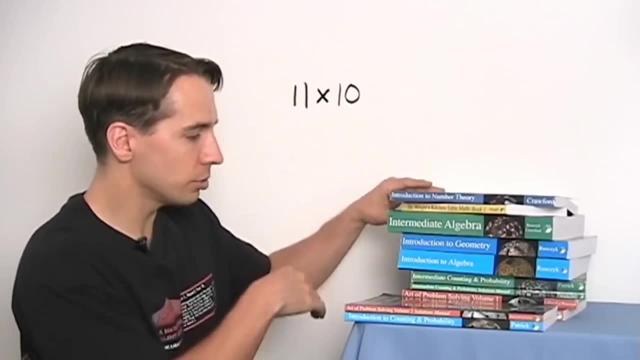 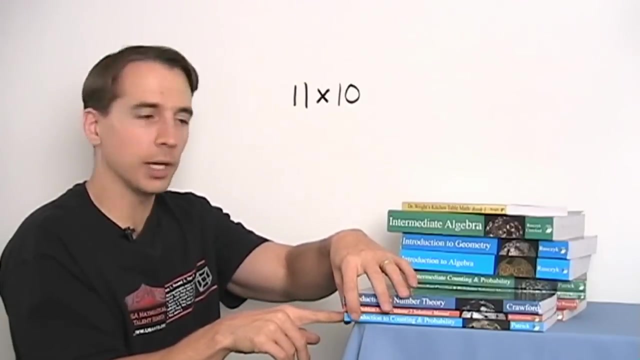 We care about the order, So these two are different. Now that we have two books out of the original eleven, we have nine left And we can choose any one of these. So for each of the eleven times, ten ways that we place two books down on the table. 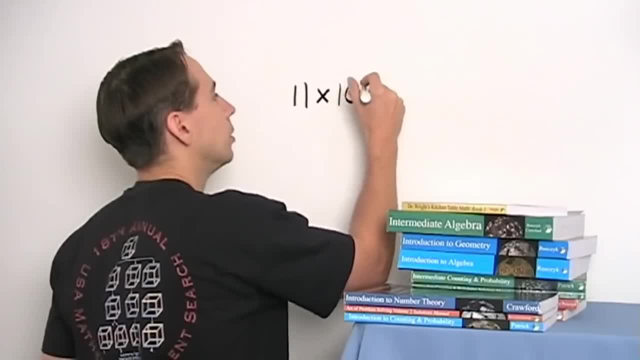 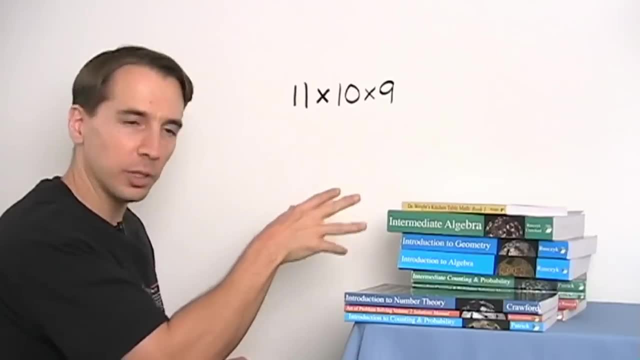 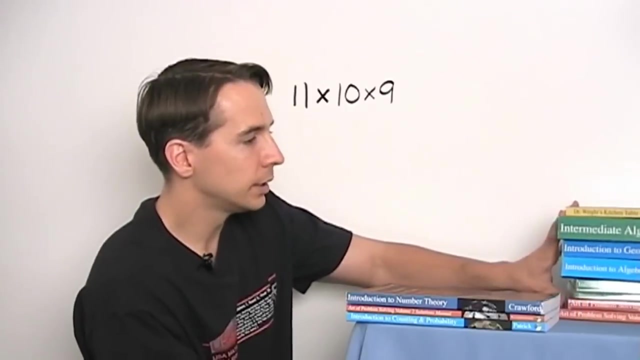 we'll have nine left, nine books left to be the third, which gives us eleven times, ten times nine ways to stack three of these eleven books right here on the table. That's great. So now I'll just push these aside And see. it's much more subtle. 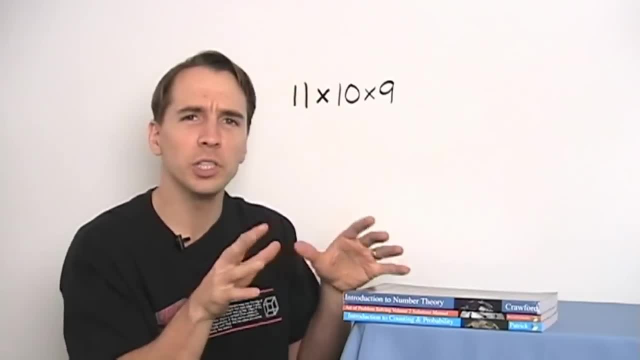 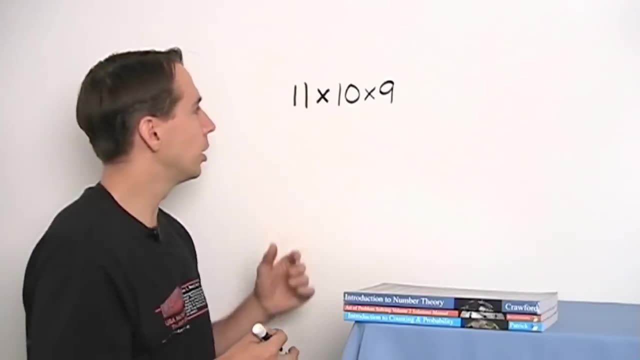 That's what they were telling me is that you'd still see the books but you wouldn't really know. you see the books And you'd remember them later And again. that's important. But even more important is that we've learned how to do kind of a new type of problem here. 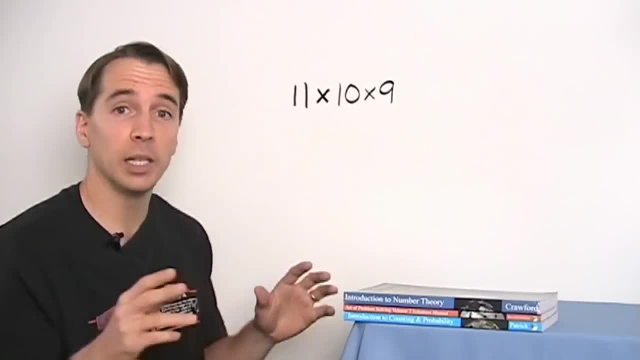 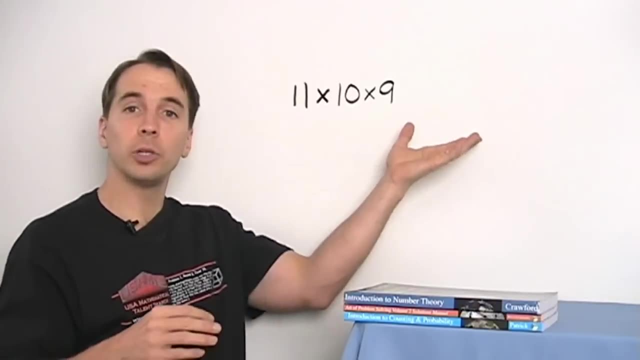 Or at least it looks like a new type of problem. It even has a new name. That name is permutation. But you can forget that name, Because this isn't really a new type of problem. It's just like the factorial problem we already did, except we don't go all the way down to one. 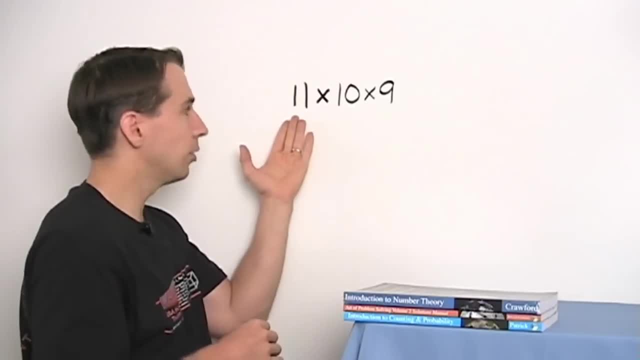 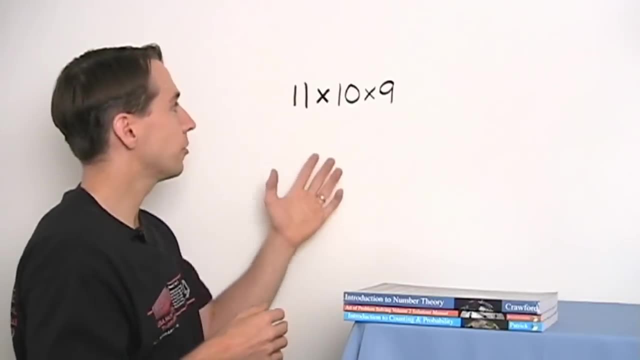 In fact, this is just a multiplication problem. We had eleven ways to choose the first book, And then for each of those eleven ways, we have ten ways to choose the next books. There are eleven times ten ways to choose the first two books. 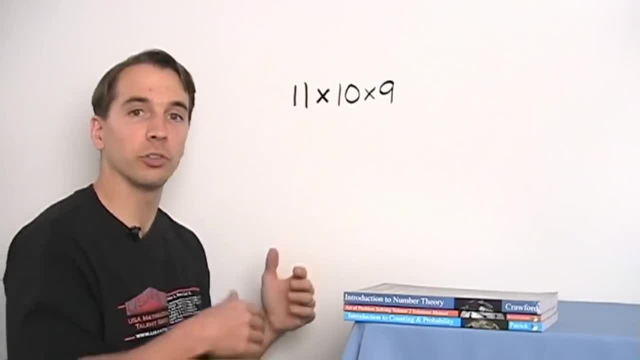 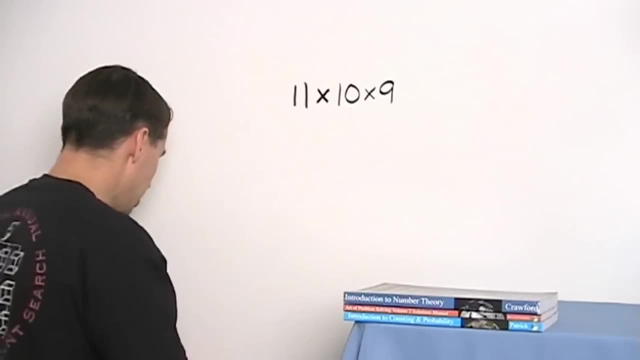 And that leaves nine books left to choose from for the third book. So there are eleven times ten times nine ways to make our stack. So don't worry about the word permutation, It's just multiplication, And make sure you understand that it's just multiplication. 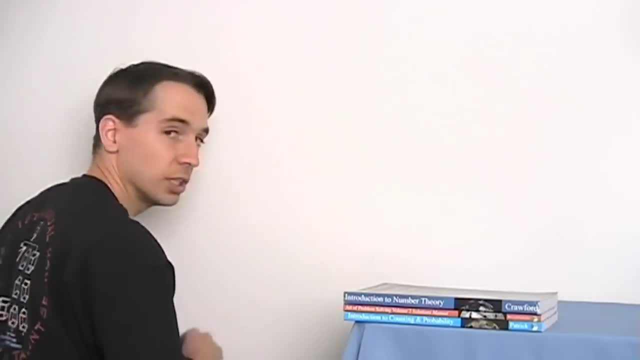 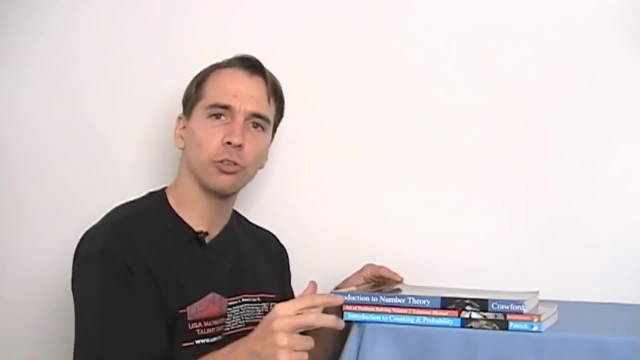 We're going to do one more problem. that not only gives us a chance to see that it's just multiplication, but also gives me a chance to tell you that we don't just have books here at Art of Problem Solving, but we also have classes. 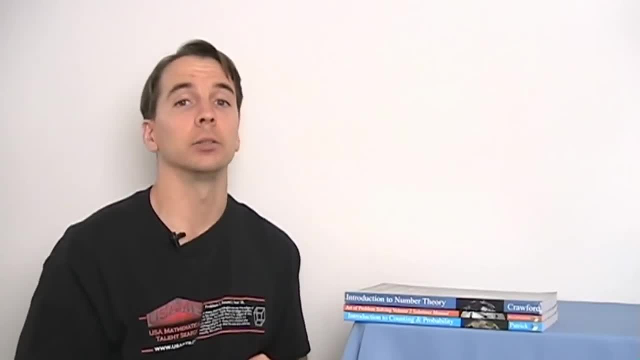 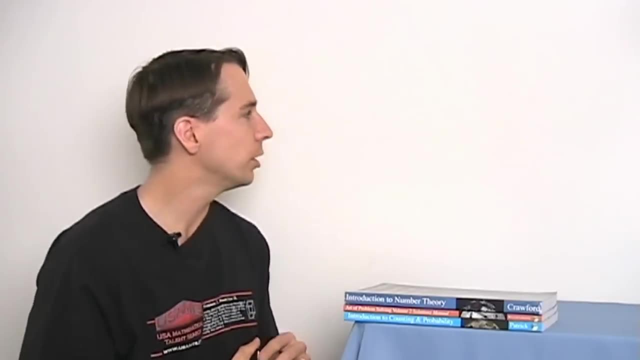 One of those classes is called the Worldwide Online Olympiad Training And that is a class for high school Olympiads, for students training for really hard problems, And you'll probably be ready for this class in a couple of years, And in this course we have seven instructors. 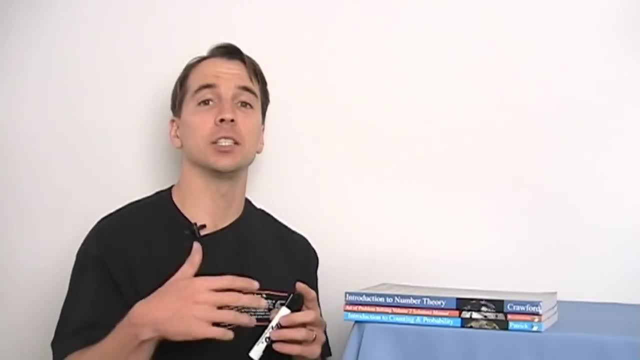 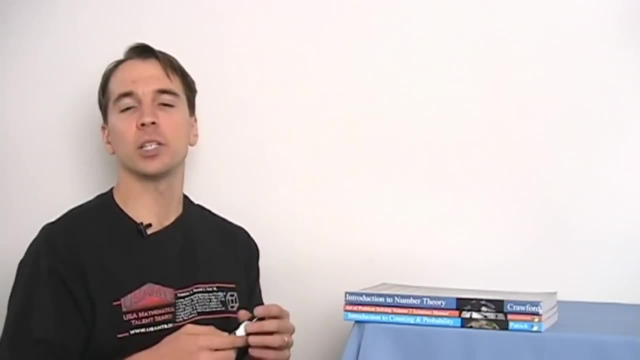 For our first four classes. we don't ever want to have the same instructor teaching two classes. We want to have four different instructors for those first four classes. So the question is: in how many ways can we assign the instructors to those first four classes? 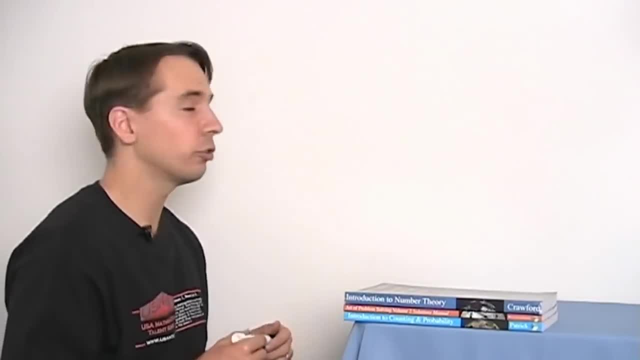 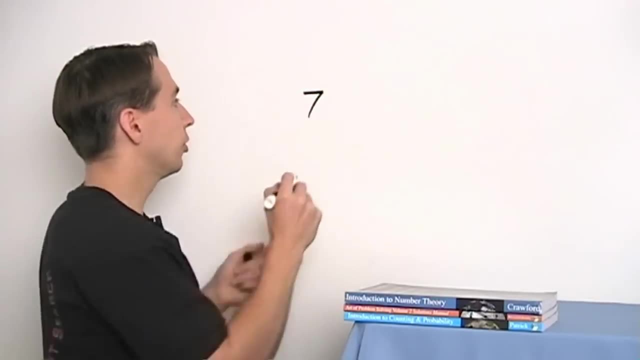 And it's a lot like the book problem. At first we choose the first instructor- There are seven ways, because we have seven instructors- And then, once we've chosen the first instructor, well, for the second class we can't have that same teacher. 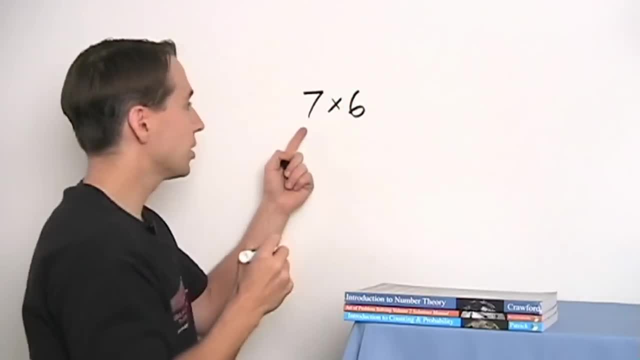 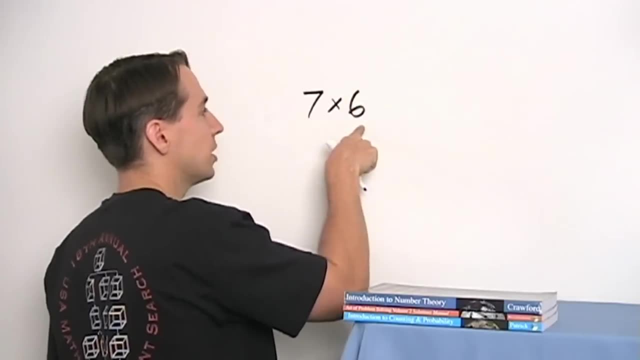 So there are now only six teachers left for the first four classes. So there are seven times six ways that we can choose teachers for the first two classes And then continuing in the same way. for each of these seven times six ways, we choose the first teachers. 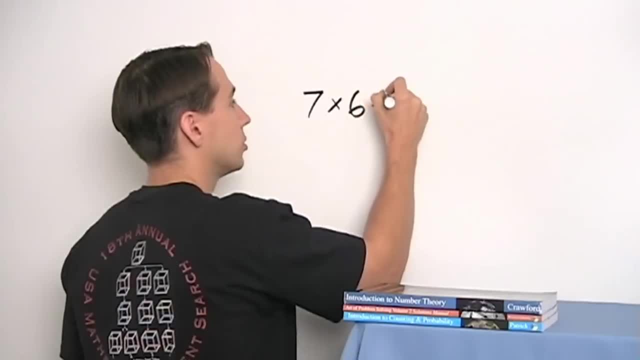 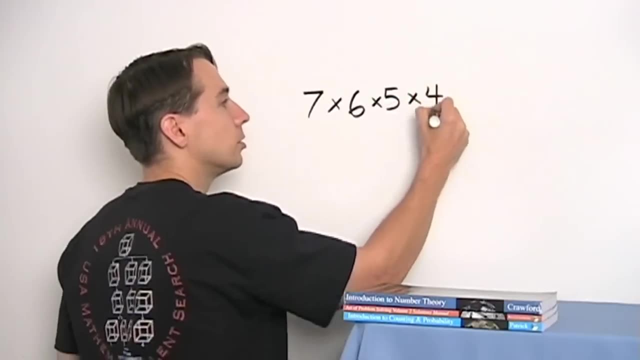 there will be five teachers left for the third class. So there are seven times six times five ways to choose our first three teachers And then on to our last teacher. we've chosen three out of the seven. That means there are four left.